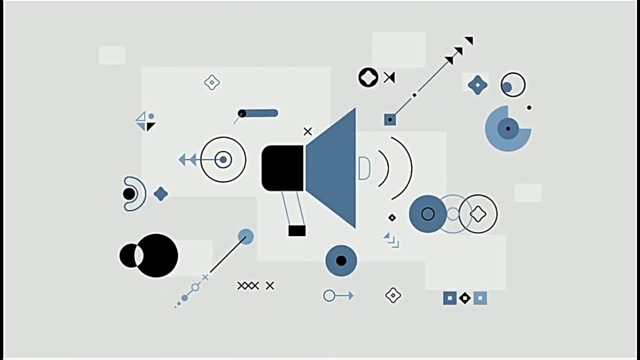 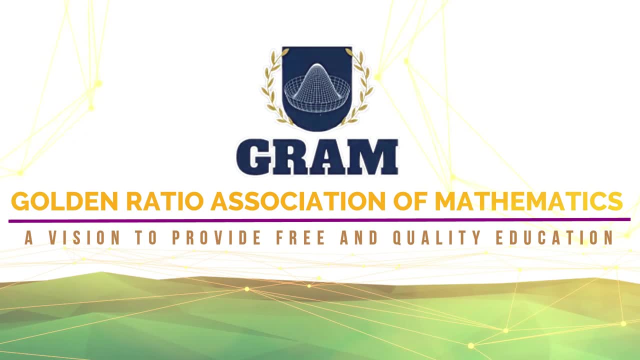 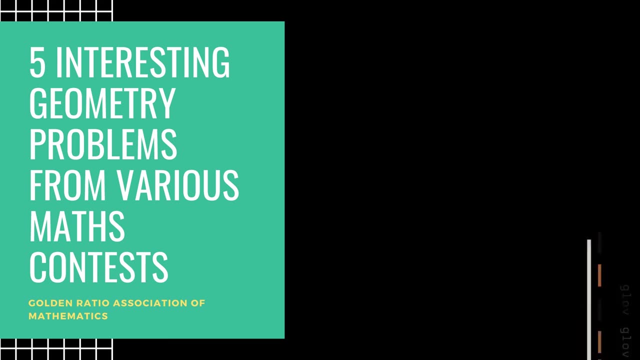 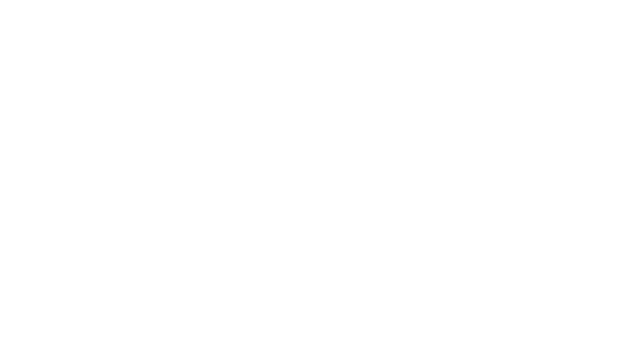 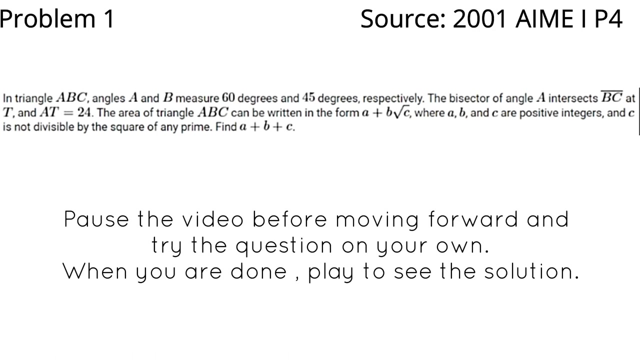 Hello everyone, welcome to golden ratio association of mathematics. I am Samar Yadav and in this video I will be sharing five interesting geometry problems from different math competitions. Solutions of these questions have been proposed by Srijan Sarkar, So let's get started. 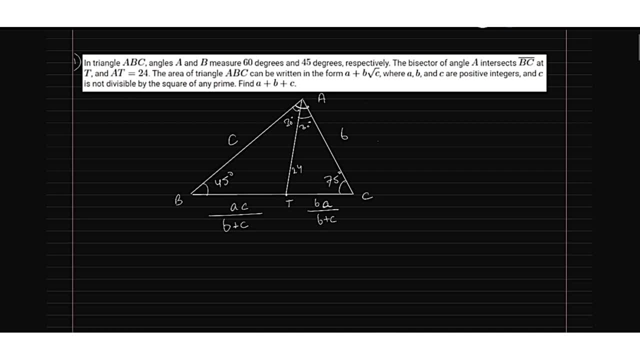 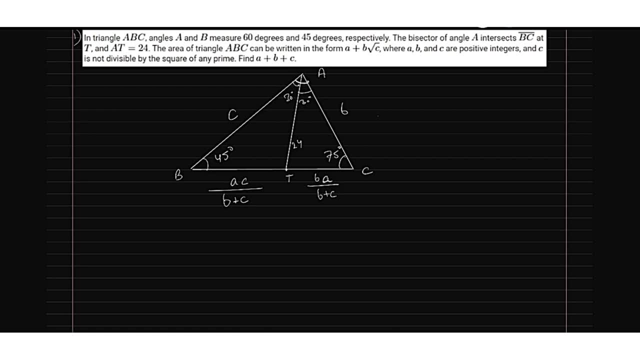 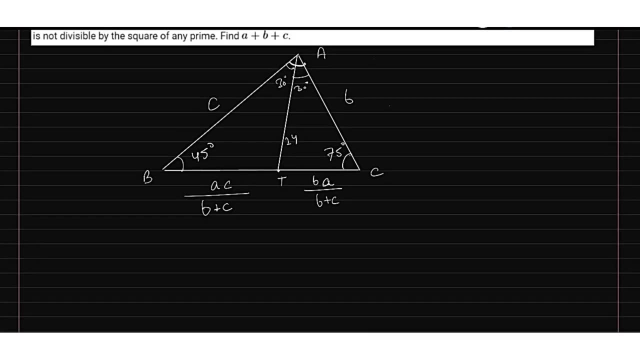 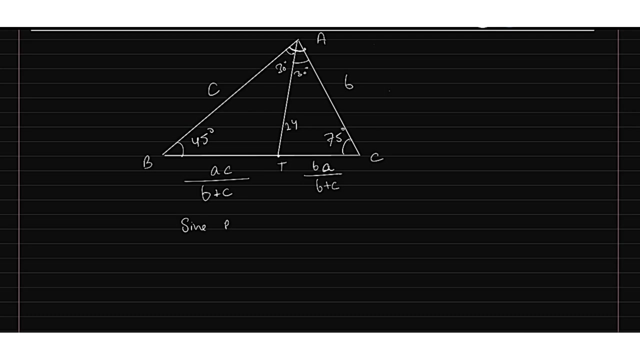 So let's start with the first question. I've drawn the figure here. Okay, I assume you have tried the question till now, So let's start start solving the question. First of all, let's apply sine rule. We'll need the need sine rule for further in the further part, So let's apply it by sine rule. 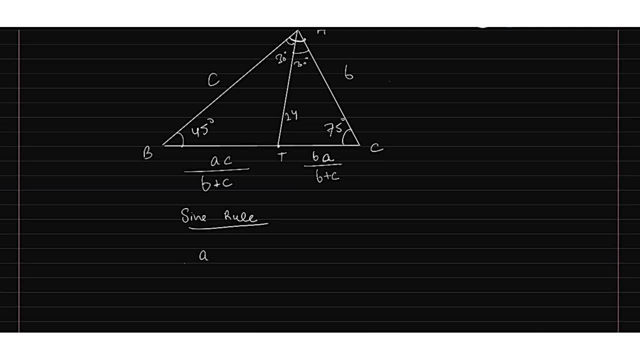 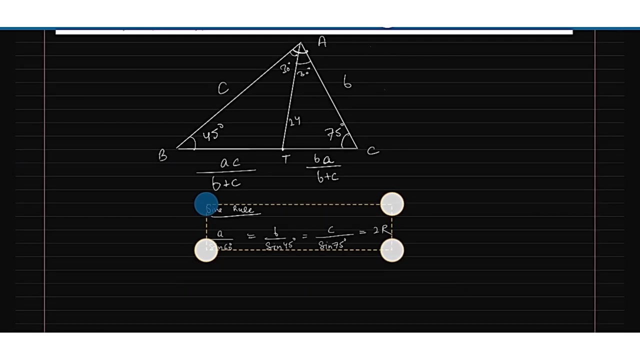 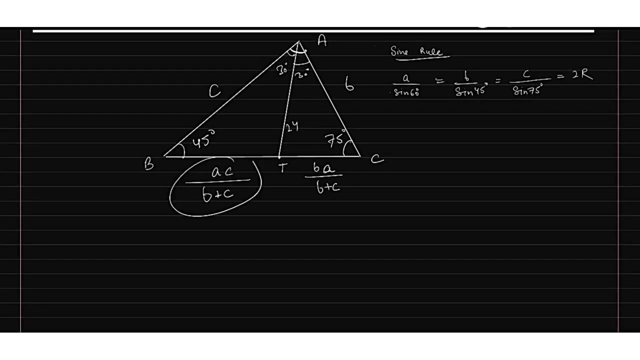 You have a over sine 60 degrees equals b. over sine 45 degrees, equals c. over sine 75 degrees, equals 2r. Let's keep this in the corner. We will require it further. I have labeled this part using the angle bisector theorem. You must know that before solving. 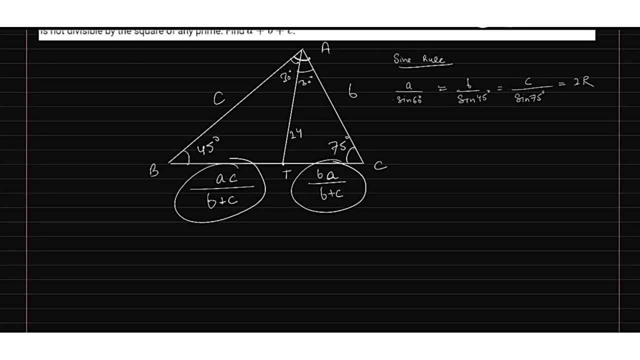 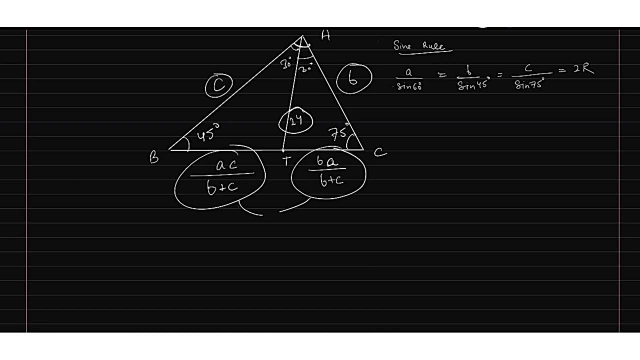 this question. First of all, we have this side, We have this side, We have these two, These have circled. We have these two and I have this. These all are the sides required for selving for Stewards theorem. 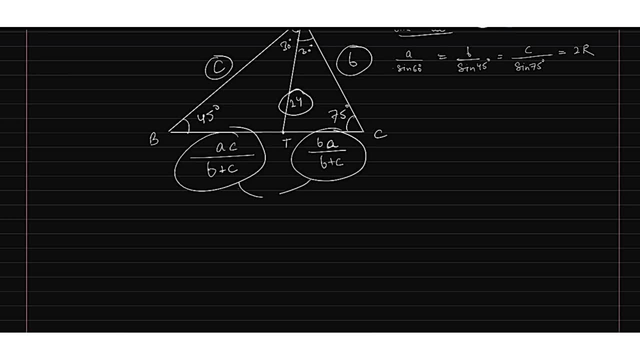 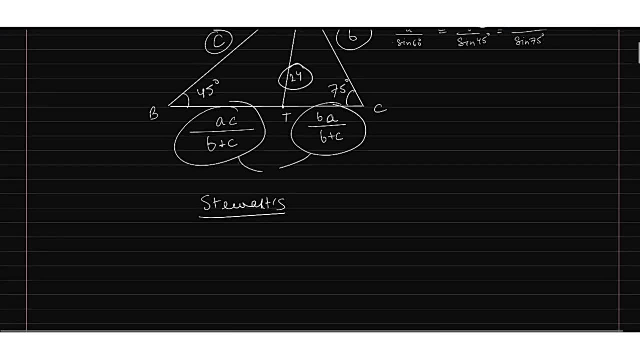 So here we get the motivation to apply Steward's theorem. So let's apply Steverts theorem. So here we have just circle under circle. That's all for now. Let's come back here before we start solving this case. This is videoじゃ y vedan c. 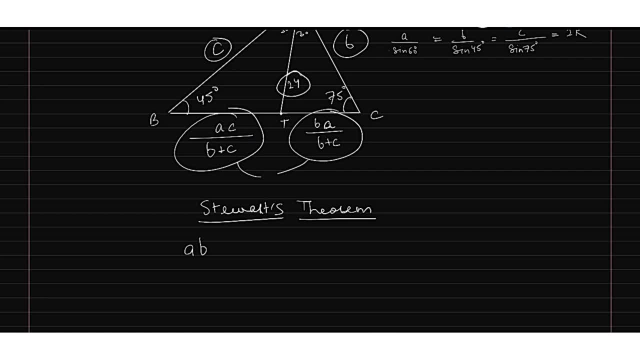 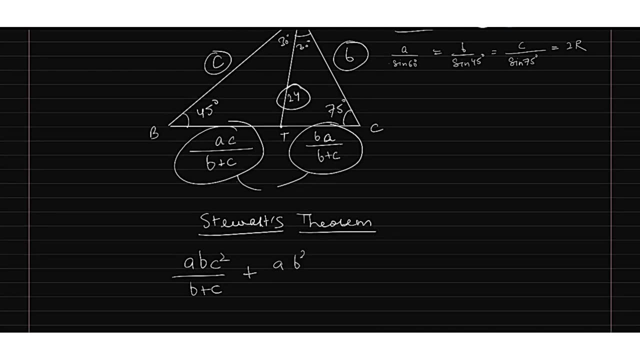 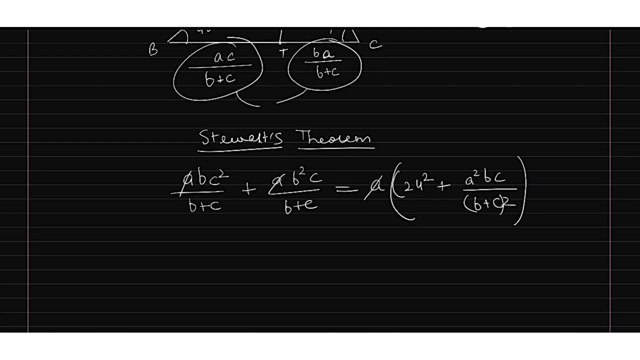 From Stewart's theorem we have ab times c square over b plus c plus ab. square c over b plus c equals a times 24 square plus a square b, c over b plus c square. Let's simplify it. We can cancel a from both the sides and take out b, c, common b, c, b over. 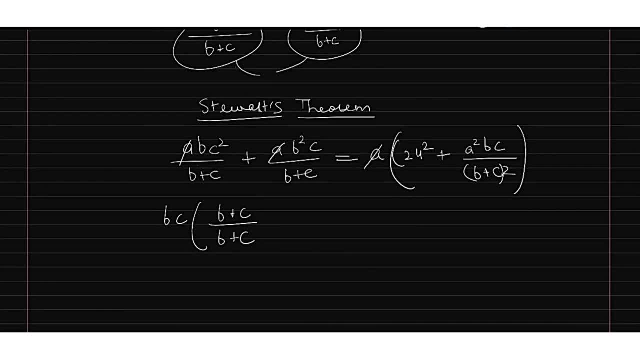 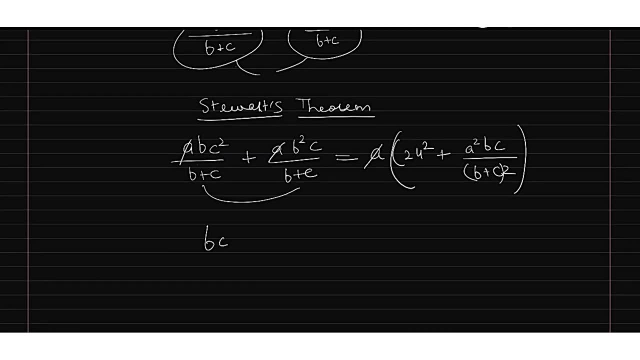 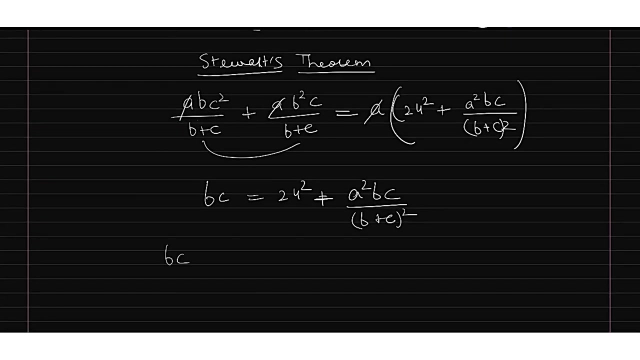 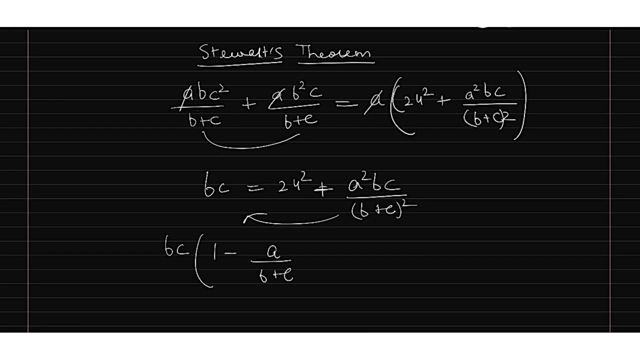 c plus b over c. This whole term equals b over c. Let me write it: b over c equals 24 square a. square b: c. b over c, b over c, b over c. let's take this term here to the left hand side: 1 minus a over b plus c, whole squared. 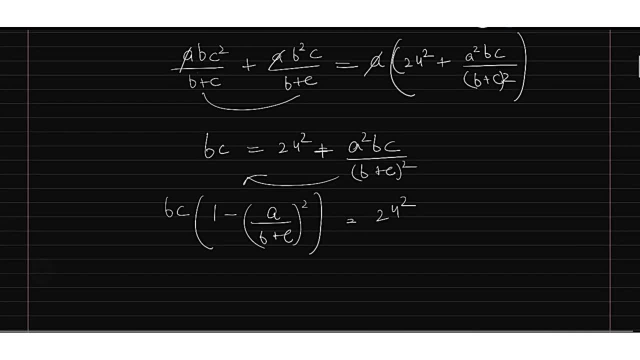 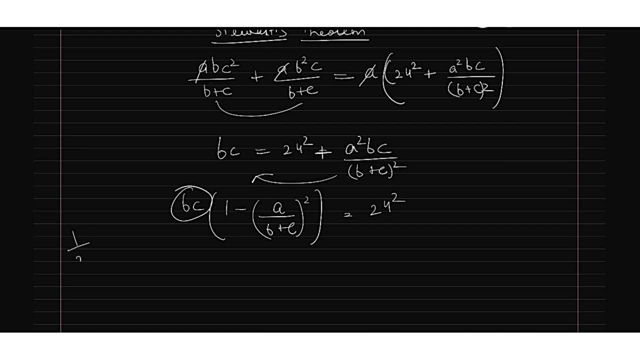 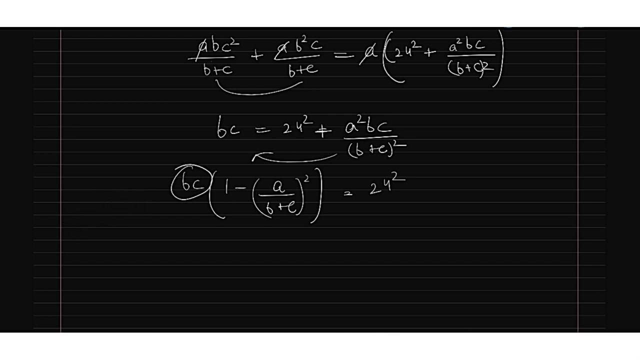 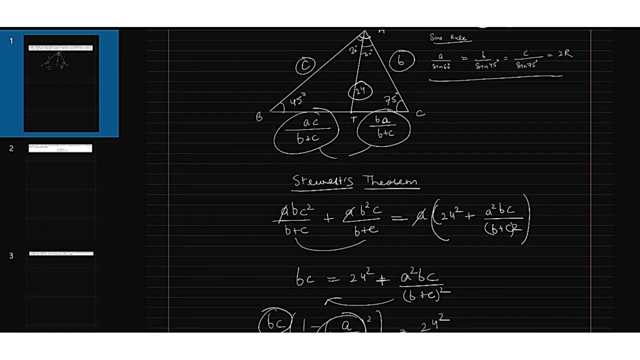 which is equal to 24 square for area. we need b c. you must know the formula: half of b c sine a. we have the angle a. we need this b c to solve for the area. so we will get b c from here, b c, and we know this ratio from the sine rule which i said you will need further. 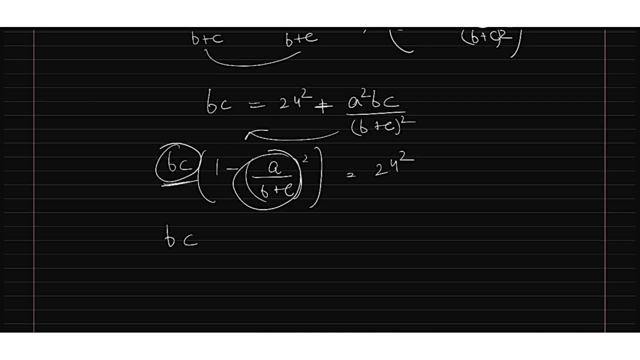 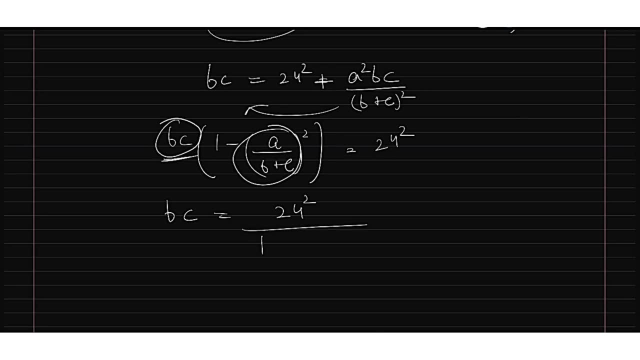 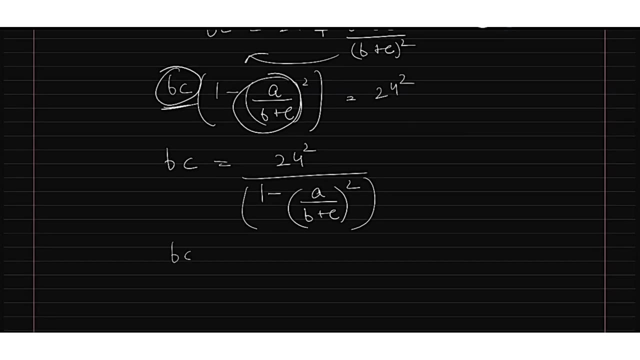 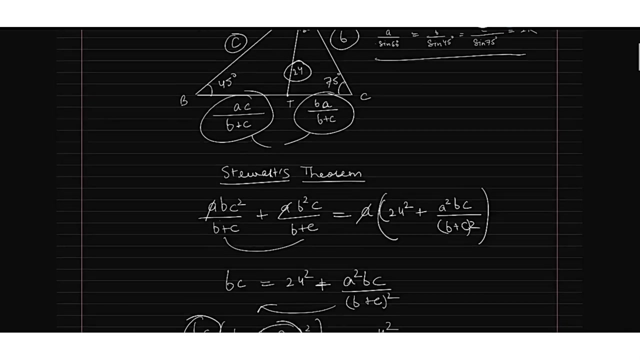 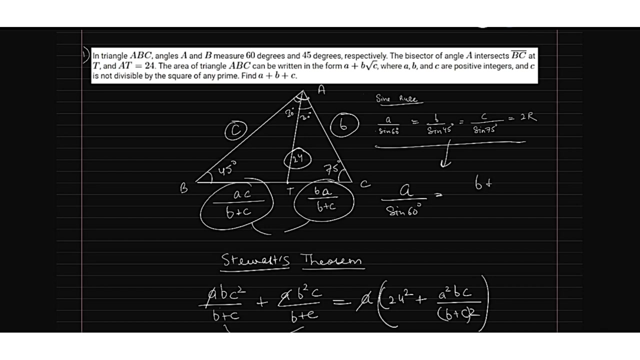 in the question. so b c is equal to 24 square over b c whole squared, which is equal to 24 square 1 minus a over b plus c. whole squared, b c is equal to 24 square 1 minus. so from here we have a sine sixty degrees equals b plus c over sine 45 degree plus sine 75. 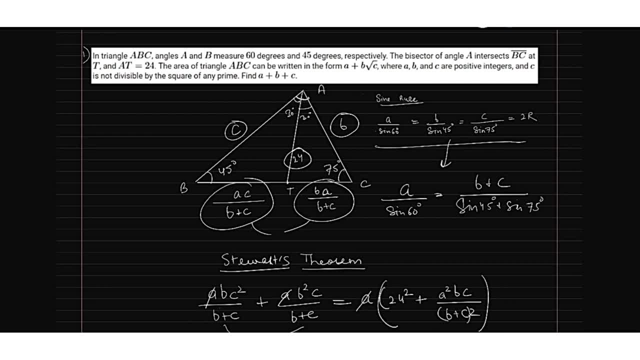 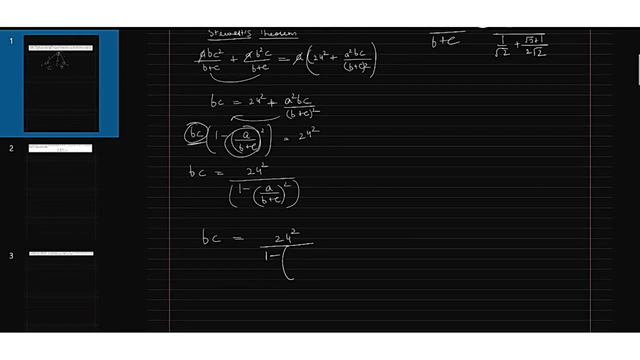 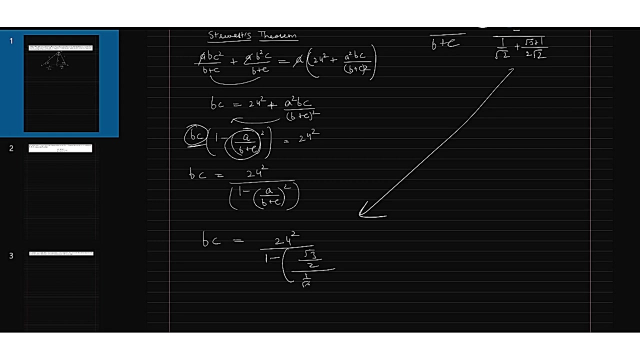 degree a times a over bc equals root 3 over 2, 1 over 2, 1 over root 2. sorry, root 3 plus 1 over 2. we can simplify this, so let's put this here: we have root 3 over 2, 1 over root, 2 plus root. 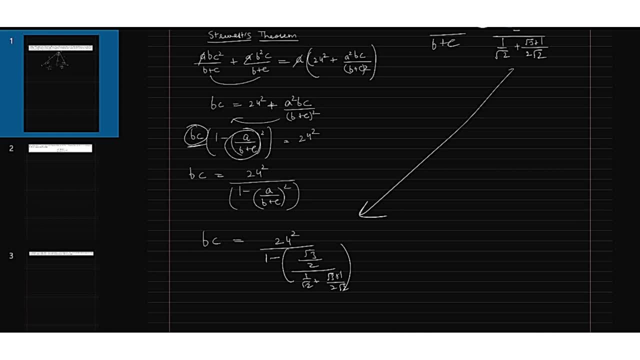 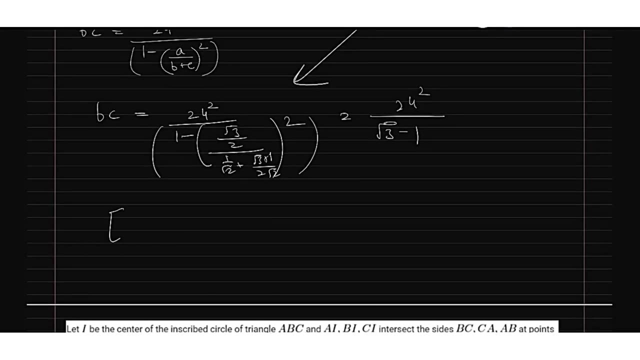 3 plus 1, 2 root 2. whole squared 24 square over. this will simplify to root 3 minus 1. so I area of a bc equals half of sine a times bc, which is equal to 1 over root 2, root 3 over. 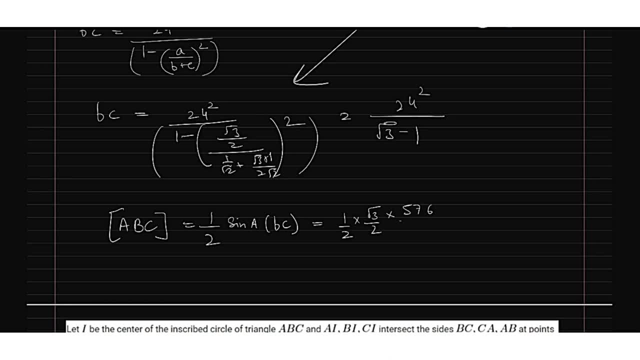 2 times 576 over root 3 minus 1. cancel from here. we will get 72 over root 3 minus 1 and cancel from here: we will get 72 over root 3 minus 1. cancel from here: we will get 72. 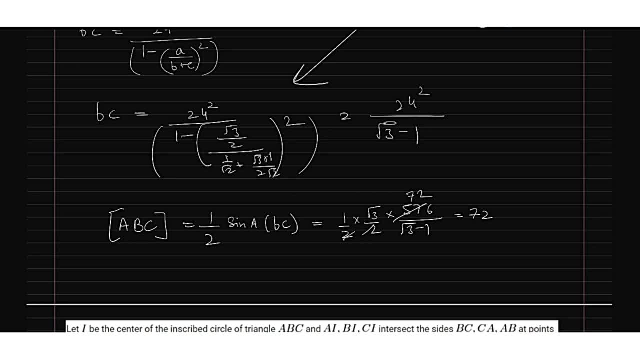 72 till you miss. will perform the values here half of rule three into the wrong three over 2 into 576, or will perform the values here half of into 576 over root 3 into root 3 over 2 into 576 over 52. 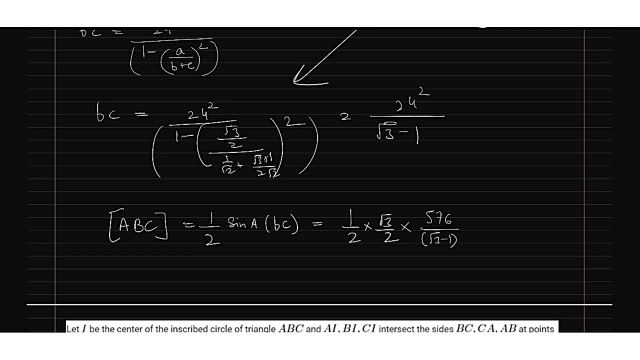 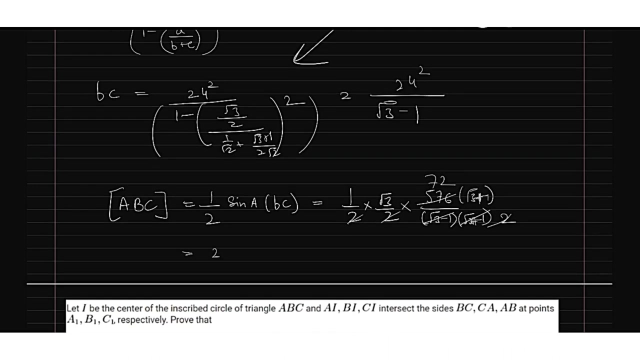 into 576 over 52, we'll be able to義. if you want to use that, you can use that. root 3 minus 1 will multiply by root 3 minus 1 and root 3 minus 1. here this equals plus 1, this equals 2 and we'll cancel all these by this and it equals. 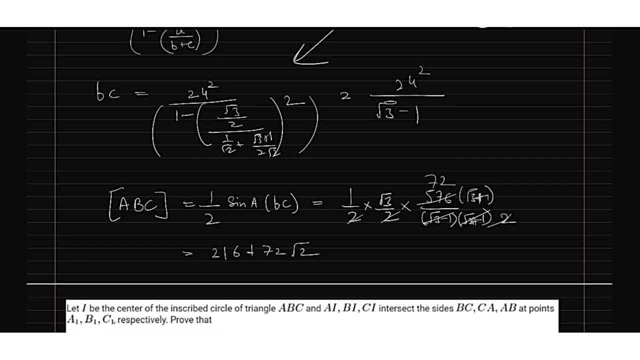 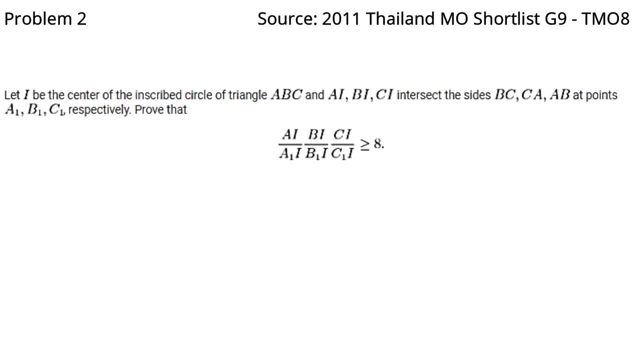 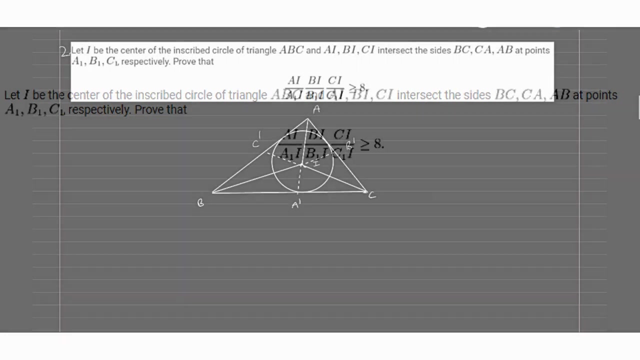 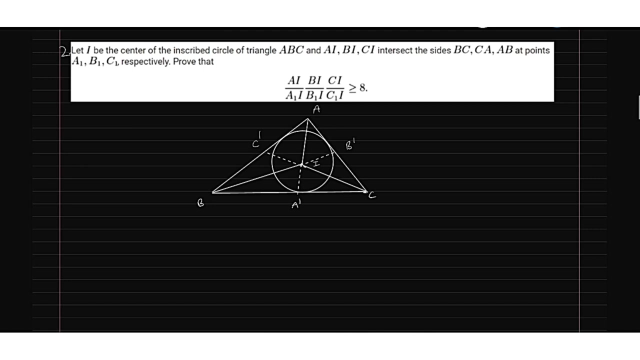 216 plus 72 root 3, so this is a, this is B, this is C. a plus B plus C equals 219. so this is our answer here. we have the second question here in this triangle, I is the in center of the inscribed circle of the triangle ABC, we have angle bisectors a, a, dash B, B, dash C. 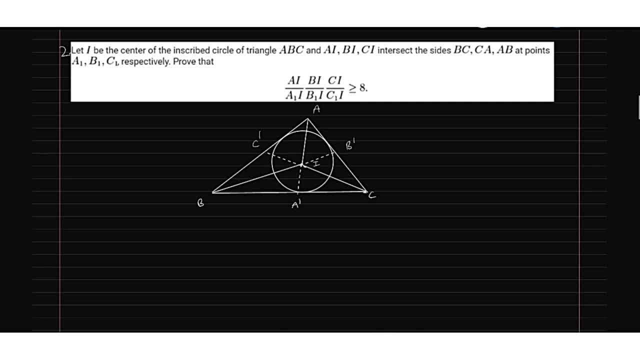 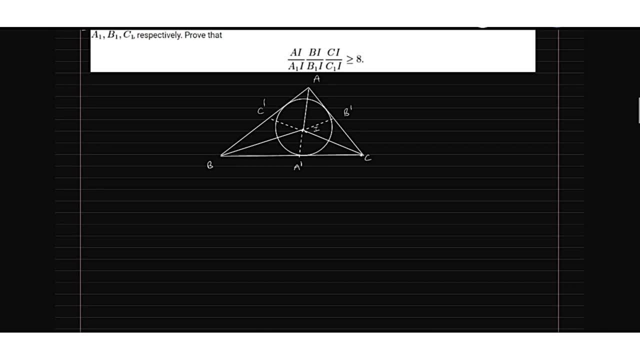 C dash, which suggest from this points. so let's start this. let's start solving the question. we can. first of all, the motivation for solving this question is the following: we can. first of all, the motivation for solving this question is: comes from this angle bisector theorem in this triangle, in triangle a, B, a dash, we. 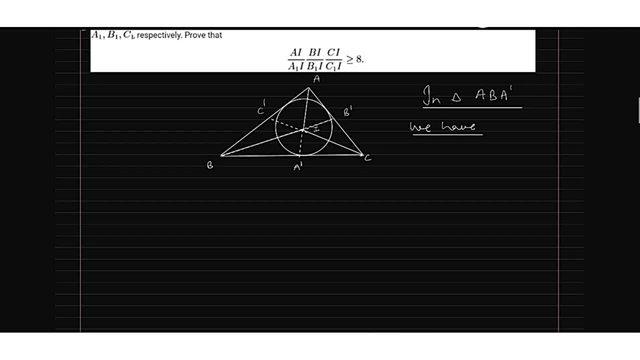 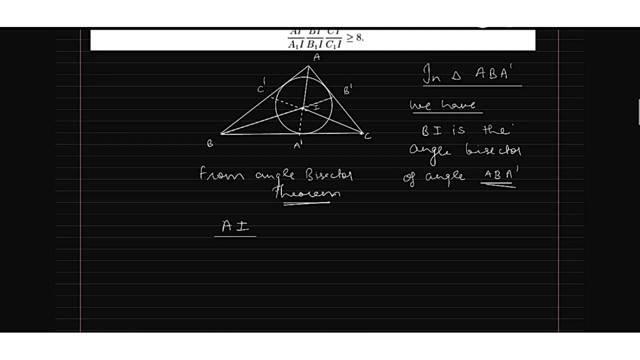 have B I, which is B. I is a angle bisector of angle a, B, a dash from angle bisector theorem B. I is a angle bisector of angle a, B, a dash from angle bisector theorem b. I is angle bisector of angle BB, a dash, B, B. we have a I over A dash I equals a, B. 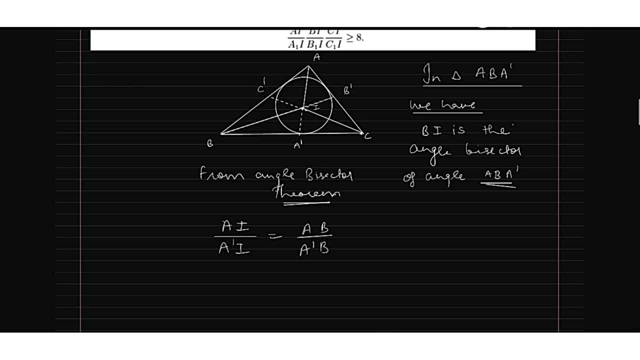 have a I over a dash I equals a B over A dash B. we have final arrival time, which is which is this length a B over this length, B over A dash B. Sма, K, Km, Km, Km equals AB over B over A dash B. 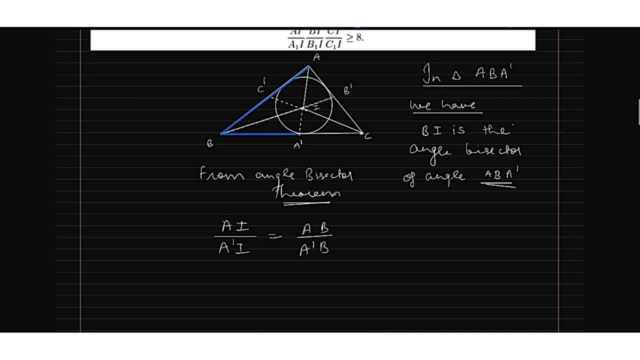 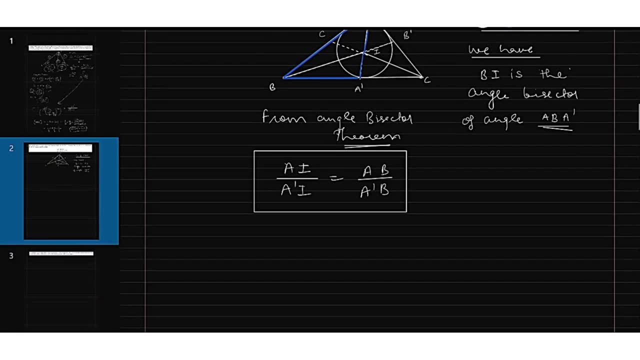 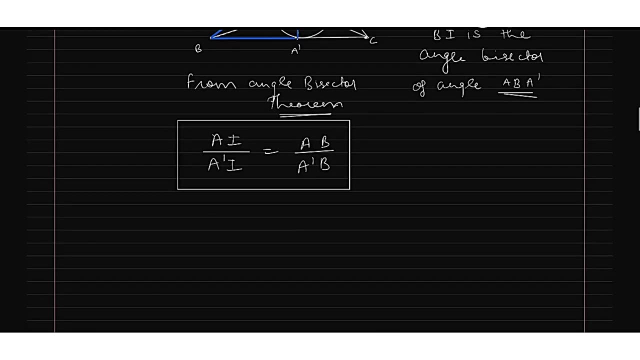 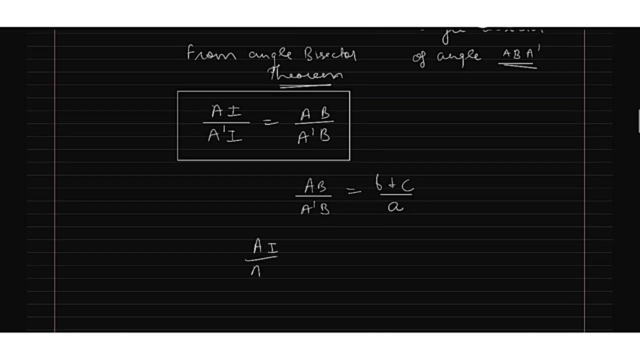 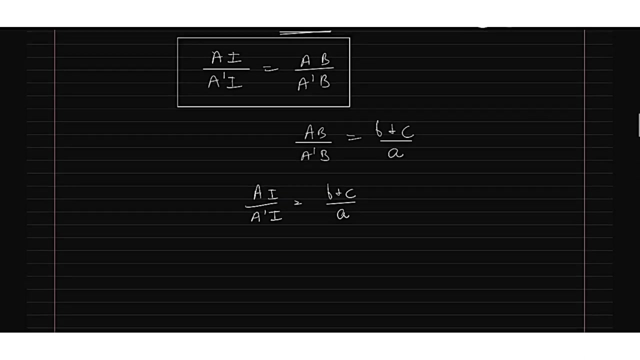 a b dash a i and a i dash. this is a result from angle bisector theorem itself. so a b over a dash b. this a b over a dash b, equals b plus c over a. so a i over a dash i can be written as b plus c over a. so our question becomes b plus c over a, a plus b over c. 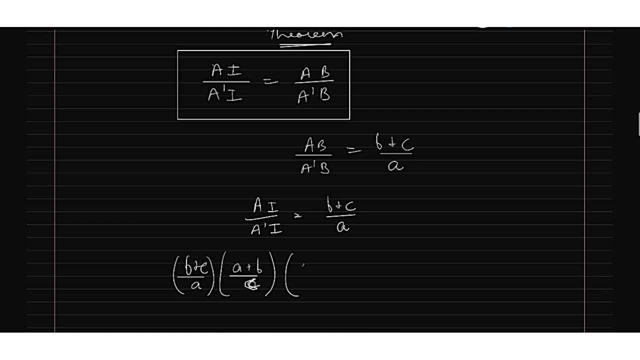 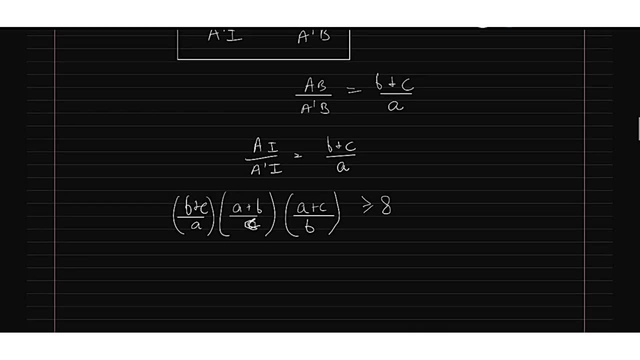 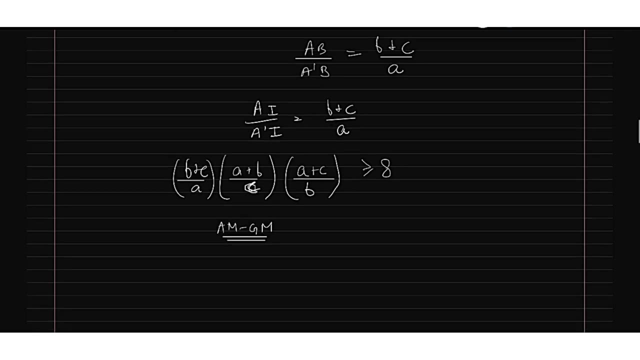 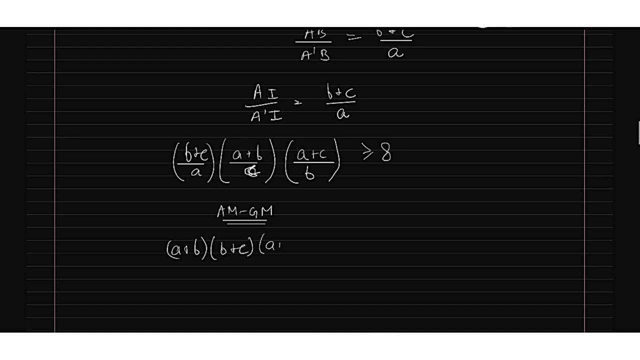 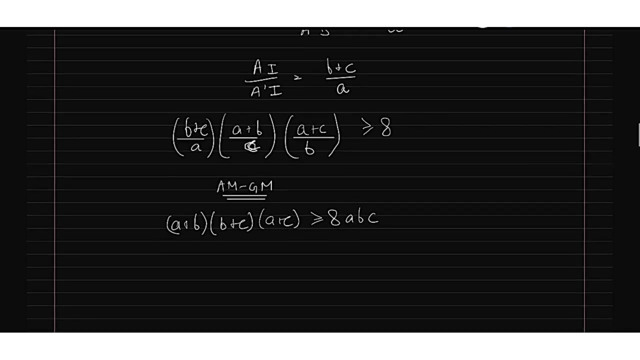 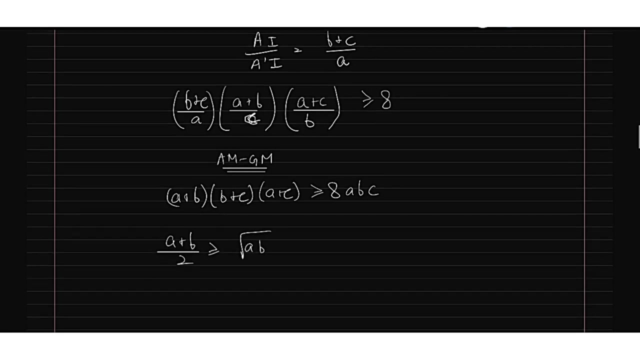 and a plus c over b is greater than equal to 8. this is very trivial from am, gm, but i'll prove it for you: a over b, b over b plus c plus c, greater than equal to a, b, c over a, c, a, t, b, c. a plus b over 2 is greater than root. ab, b plus a over 2 is greater than root. 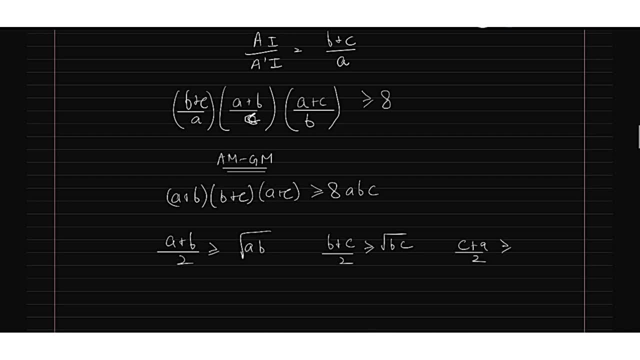 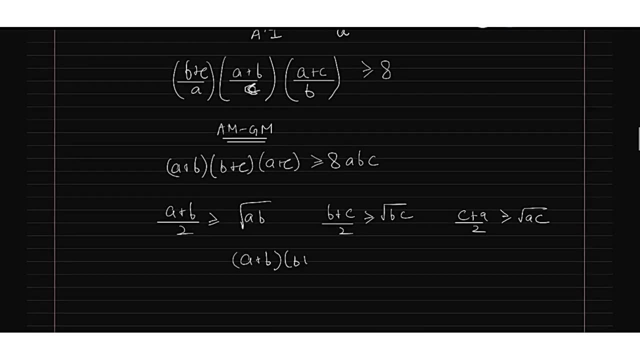 bc. c plus a over 2 is greater than root ac. we'll multiply all of these: a plus b times b plus c, times c plus a is greater than equal to a plus a, b plus a over 2 from here: okay, adding anski: Harriet, please try and do it actually. 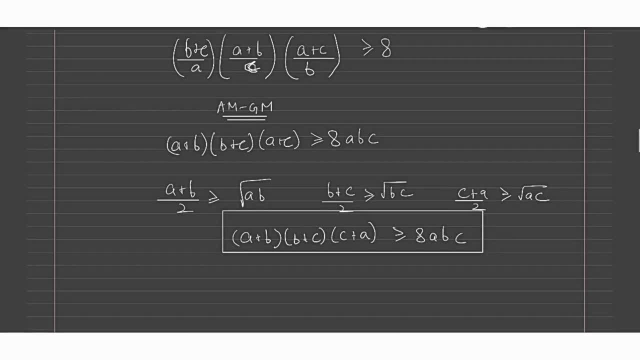 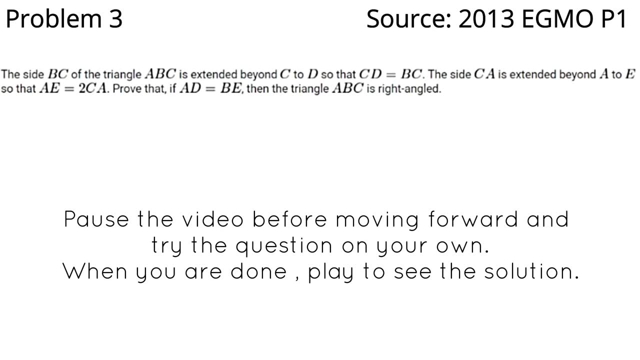 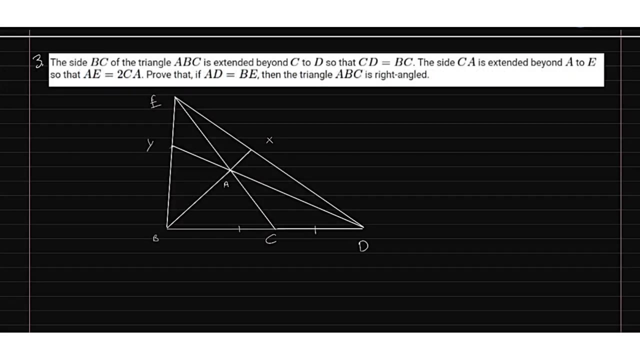 ABC. this is the result we had, which we had to prove. let's start the third question. in this question we have side BC of the triangle ABC extended beyond C to D so that CD equals BC. the side CA is extended beyond a to e so that a e equals to CA. so in this question we have extended be. 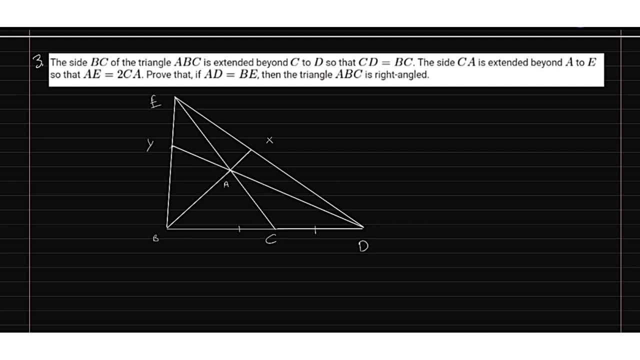 e and ad to meet at y and ba and de to meet at X. so we have these two and we have created this triangle be. e and ad to meet at y and ba and de to meet at x. so we have these two and we have created this triangle be. 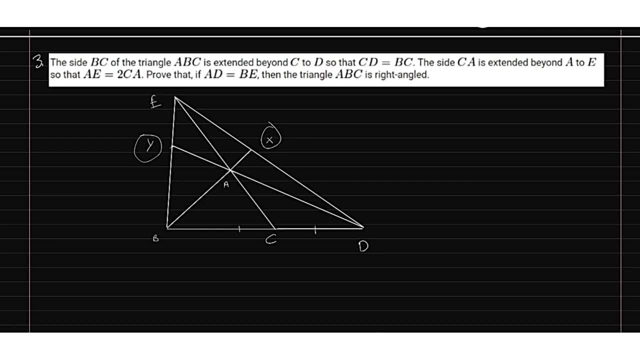 e and ad to meet at y and ba and de to meet at x. so we have these two and we have created this triangle: be e and ad to meet at x. so we have these two and we have created this triangle: be e and ad to meet at x. so we have these two and we. 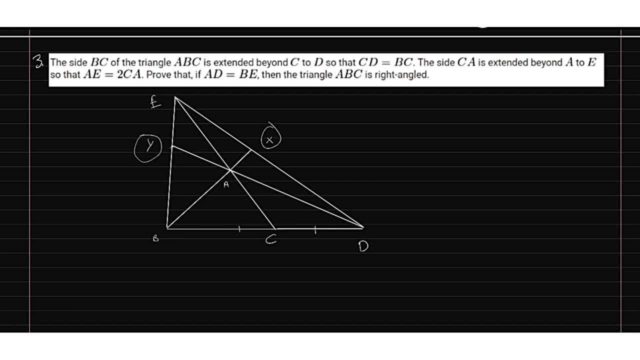 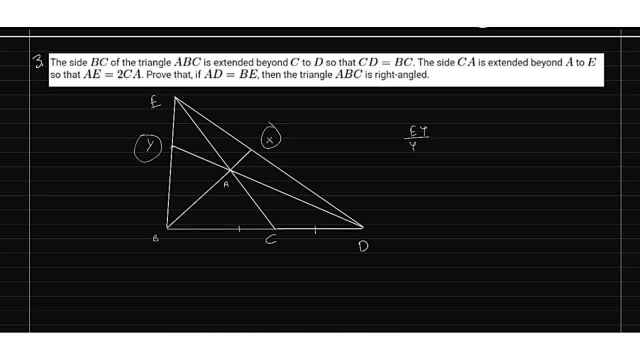 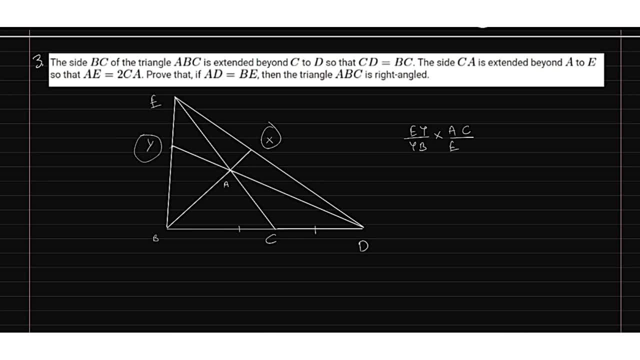 have created this triangle: be over EA times BD over CD equals 1 in this equation. we have this ratio and we also know this ratio, so we can find the ratio EY over YB- sorry, EY over YB- is equal to 1- into CD over BD, CD over BD, which equals 1 over 2, and EA over AC EA. 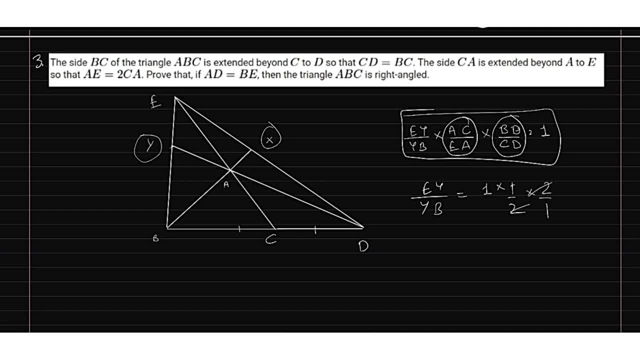 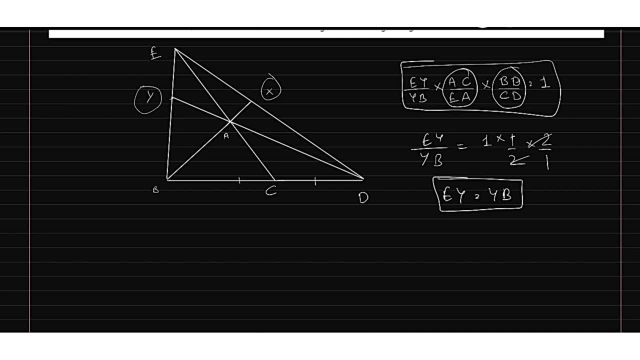 over AC, which equals 2 over 1. so EY equals YB. similarly, we can show that XD equals XC. we have this, this, this, all are equal. so a is the centroid of the triangle, B ed. also. we want to find the ratio ee, D over a. if a way, this is way. so 1, this is also 2. 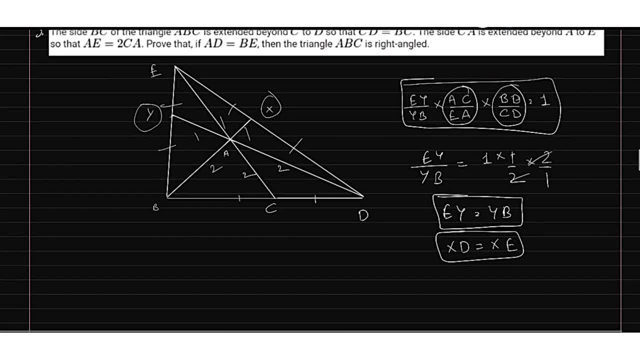 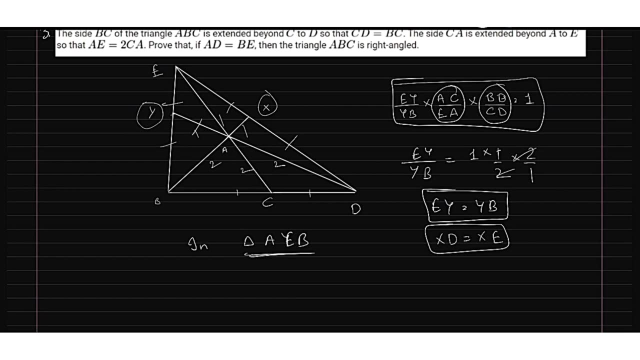 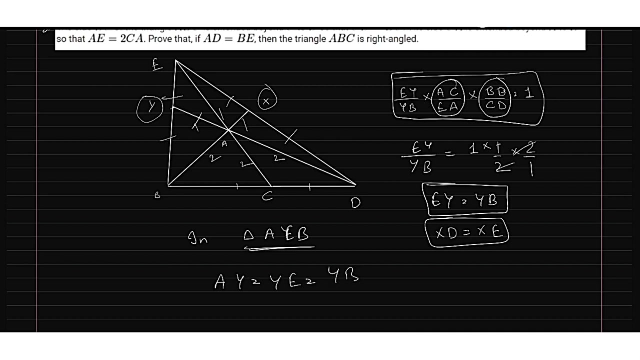 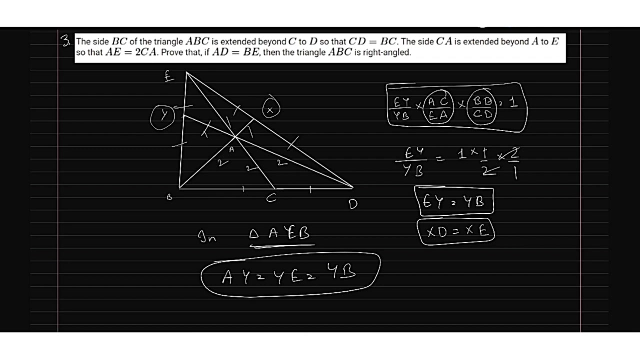 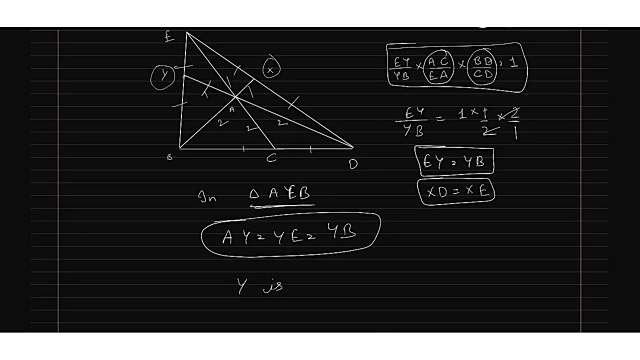 ratio 1. this is also 2 ratio 1 in this triangle, in triangle a, a, y, z, 3, 4, 5, AB, we can see that this ratio a y equals y, e equals y, B. we can notice that clearly that these three are equal. so why is the circum center? why is the? 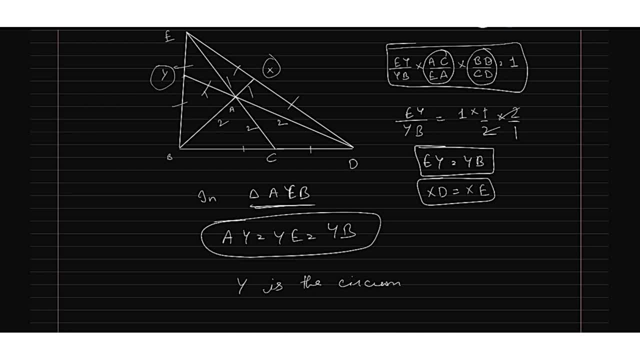 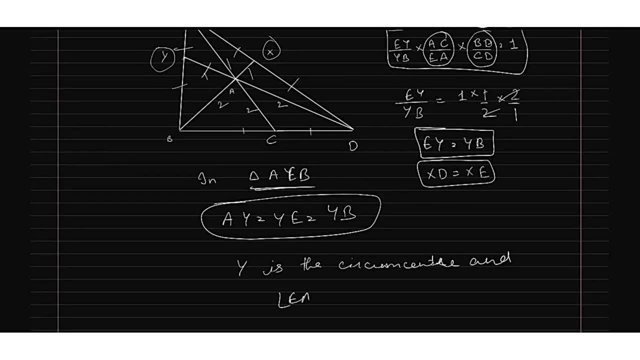 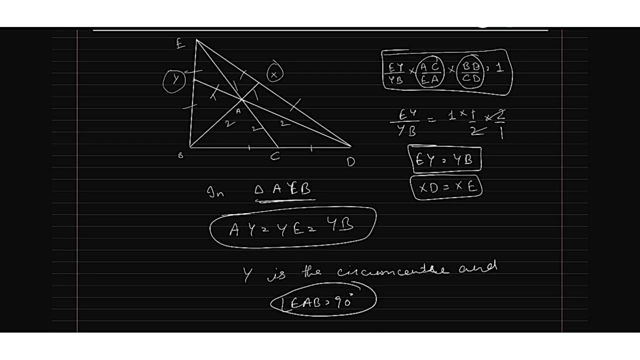 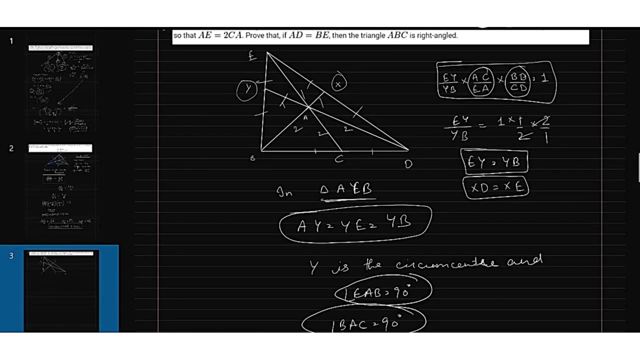 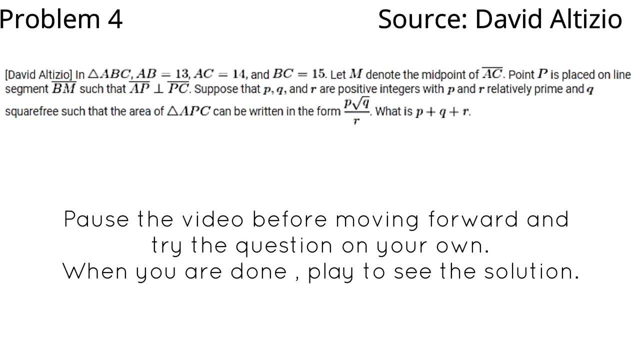 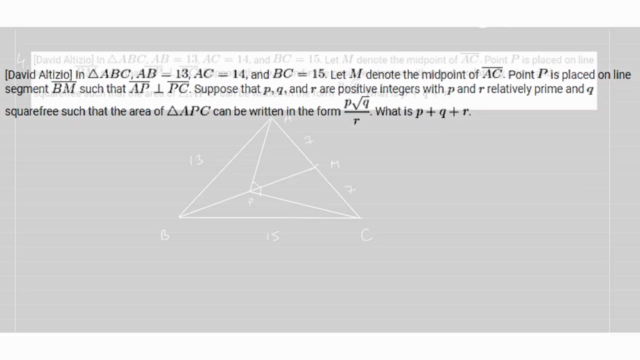 circum center and EAB equals 90 degree. so if EAB equals 90 degree, we have BAC, also 90 degree. so this proves our question that ABC is a right angle triangle. so let's begin the fourth question. in this question we have been given a 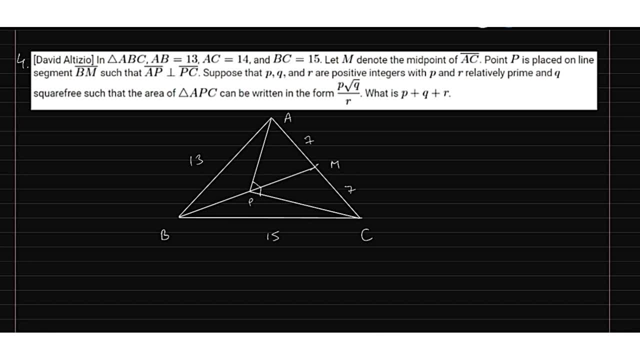 triangle ABC, which in which AB equals 13, AC equals 14, BC equals 15. let M denote the midpoint of AC. we have M here. point P is placed on the line segment B, M, such that AP is perpendicular to PC. we have AP perpendicular to PC here. 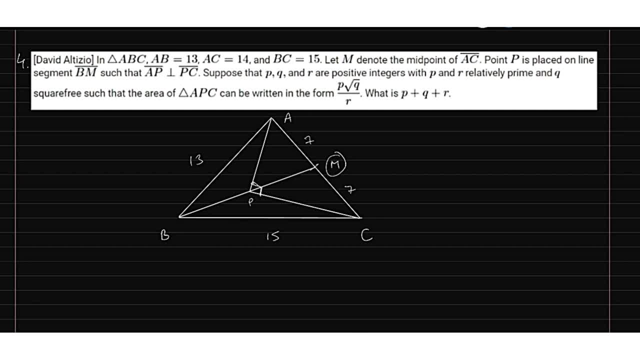 suppose that PQ are positive integers with P and are relatively prime and Q square free, such that area of triangle APC can be written in the form P under root, Q over R. what is P plus Q plus R? so let's begin this question. first of all, in this question we should 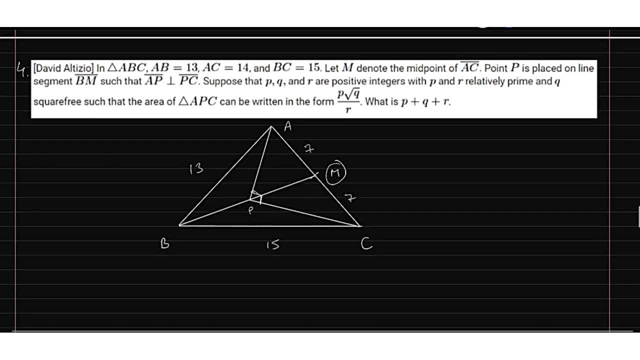 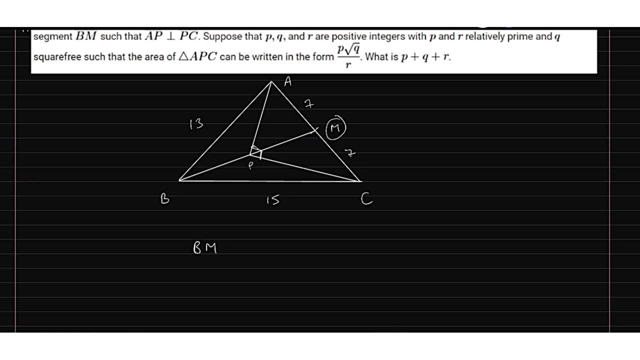 require the length of BM. we can calculate left end Canon 4 x center BN by Stewart's theorem. BM we can decorate by a Stuart serum b in. we can calculate by Stewart's theorem. we have this, yeah, this, we are just, we have this. so BM, i'm writing directly: B הפ x, Ph2. and CC our last variable there you need change your number so when producing cathedral is 28 in p1 have lm was powerful enough if there is any problem if you wanna this ​ I'll go again to the next link for this part of the video on converting the breadth of the 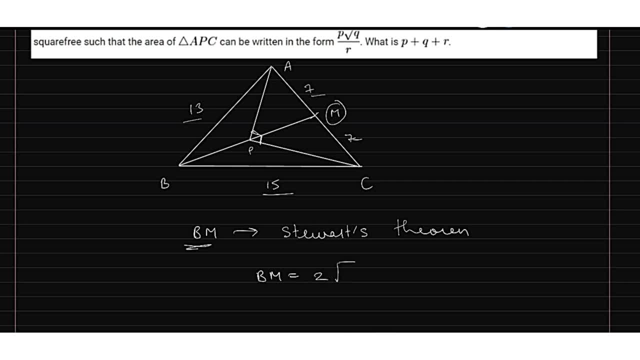 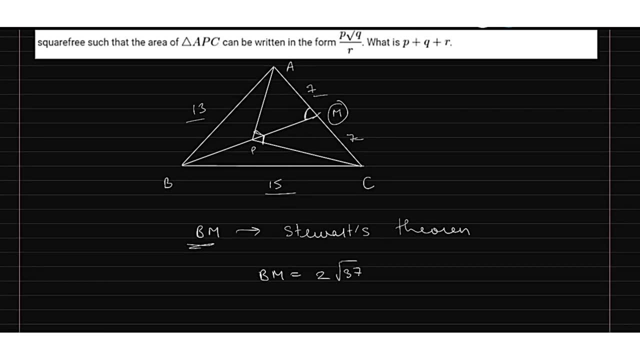 chs area members. three termifter equation is состояни Falcon America M by C plus R這個 equals 2 under root 37, so we also require this angle. let it be alpha, let this be beta, or you can write 180 minus alpha only. so cos, alpha by cosine. 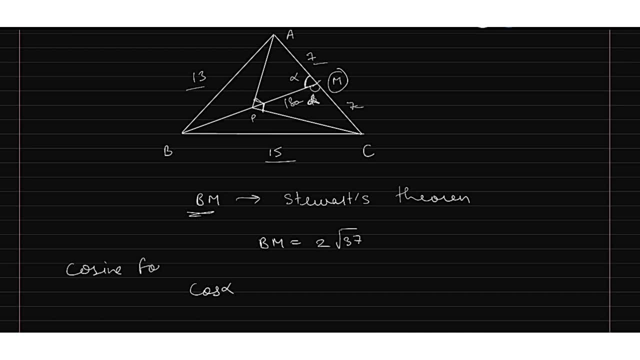 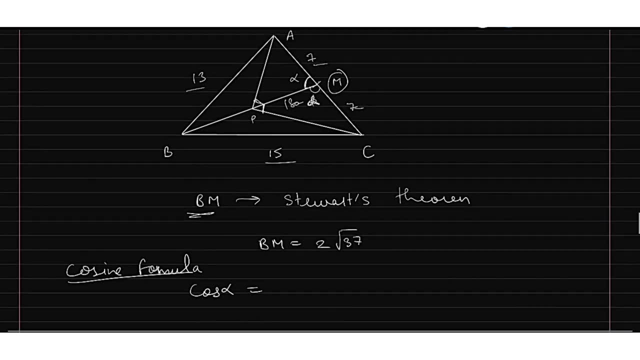 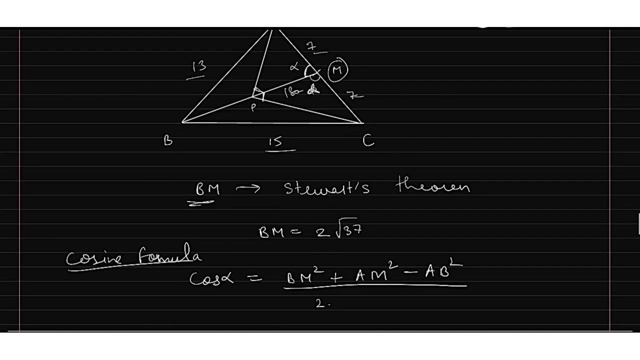 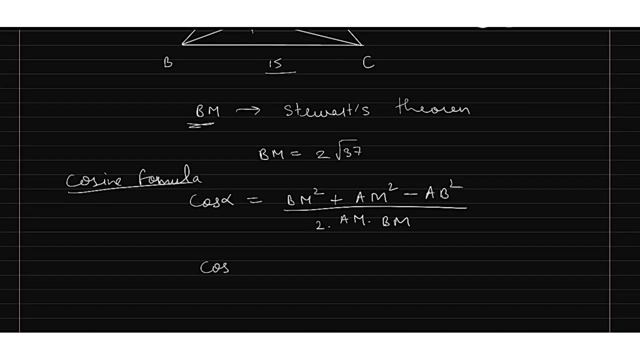 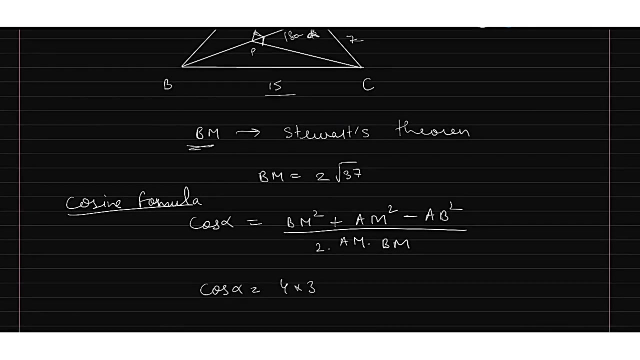 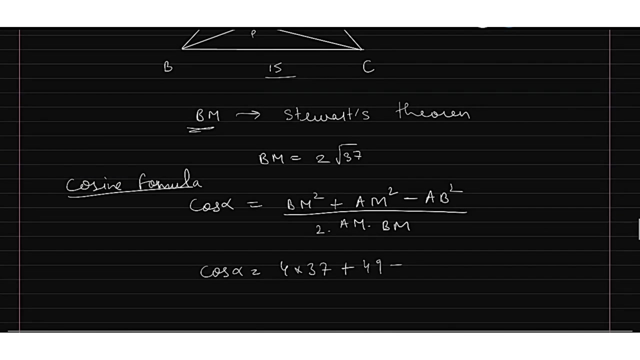 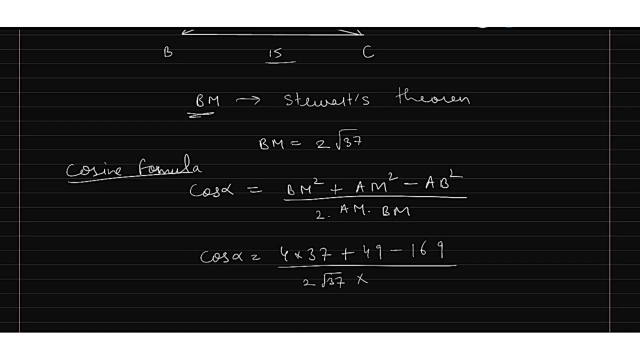 formula cosine formula: cos alpha equals bm square plus a m square minus a b square over 2 times a m times bm. we have cos alpha equals bm. we have 2 root 37, which will be 4 into 37 plus a m. we have 7. so it is 49 minus 169 over 2 root 37 times bm. we have a m, we have 7. 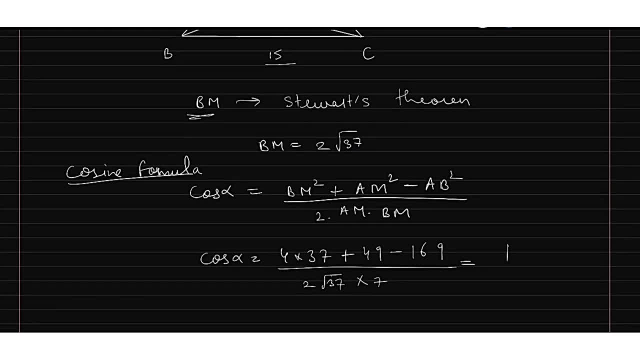 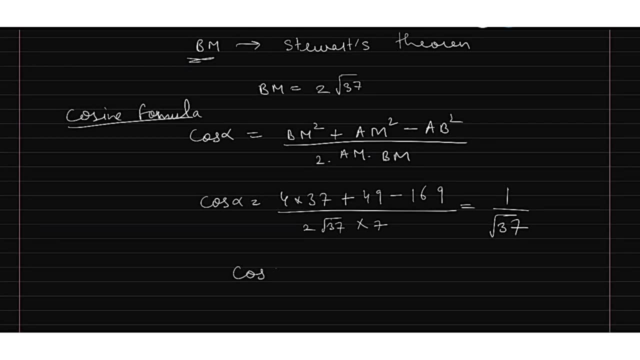 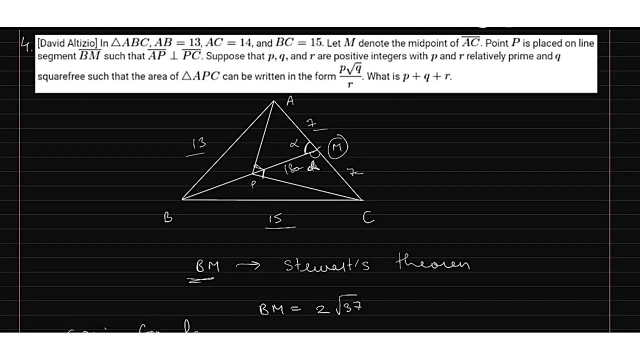 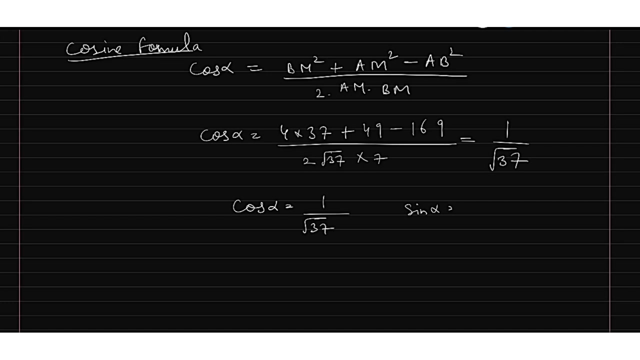 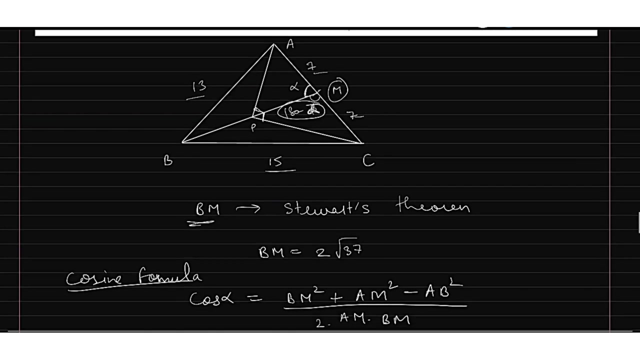 it will be simplified to root 37, so cos alpha equals 1 over root 37. as you know that we require sin alpha for calculating areas, so we'll calculate sin alpha equals 6over root 37. we can find sin beta, to which will be equal only. 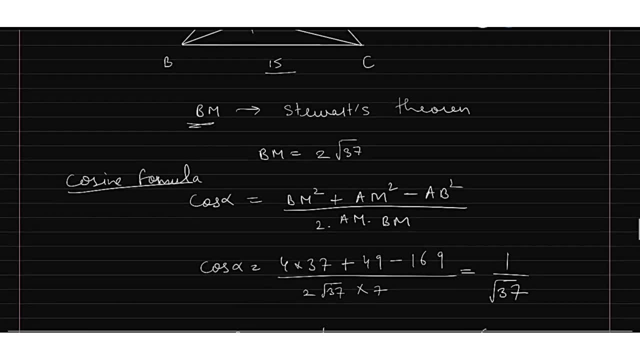 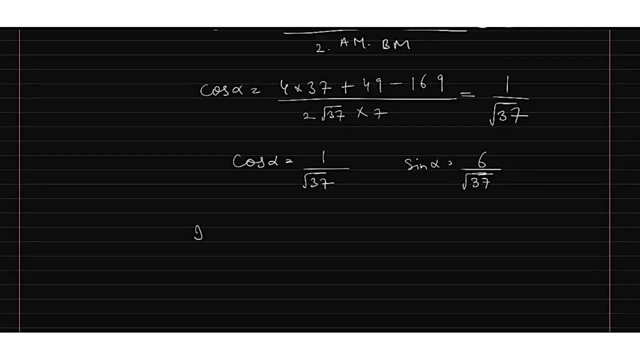 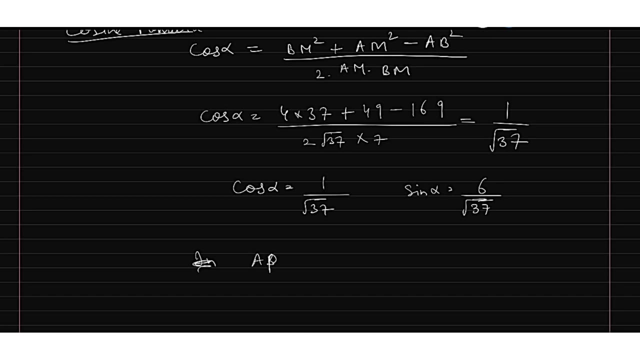 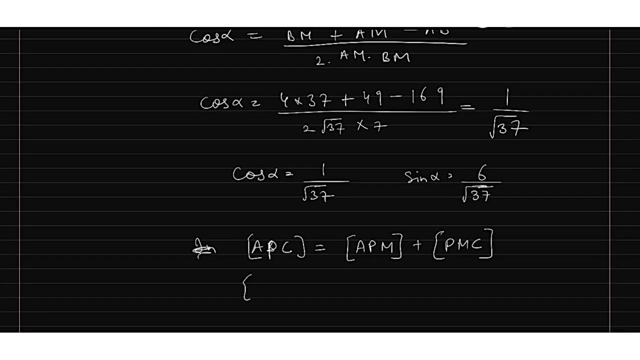 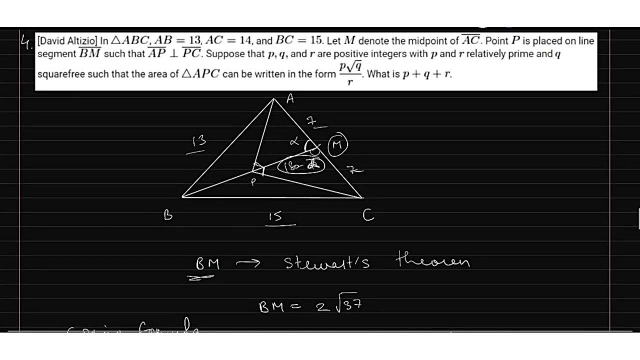 So I'm not including negative values, as these all are less than 90 degrees. So we will calculate the area of APC by: APC equals area of APM plus area of PMC. Area of APC equals area of APM. So in this triangle we have 7,, 7, so PM will also be 7.. 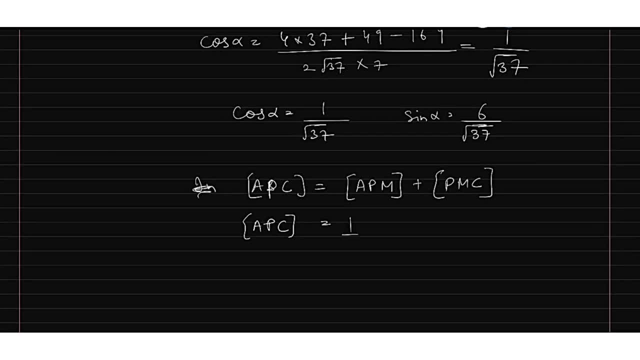 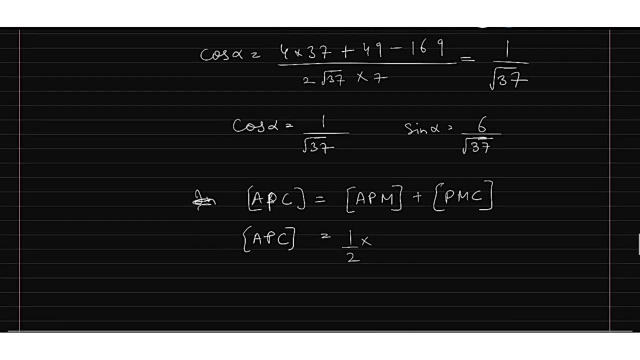 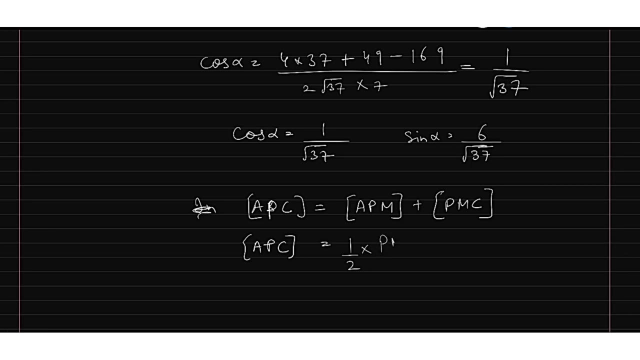 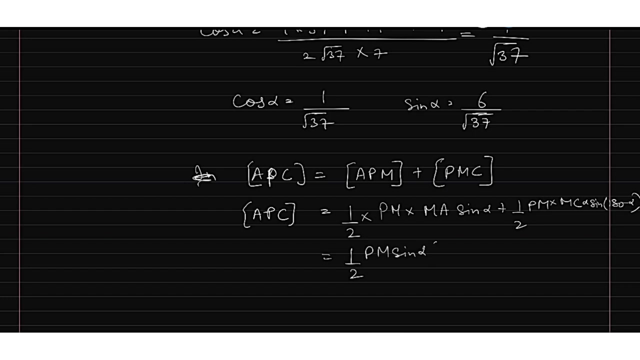 We will note that, and from the area of triangle, half BC sine alpha. we can calculate it: It is half of PM PM into MA sine alpha, plus half of PM into MC sine 180 minus alpha. Half of PM sine alpha we can take common. 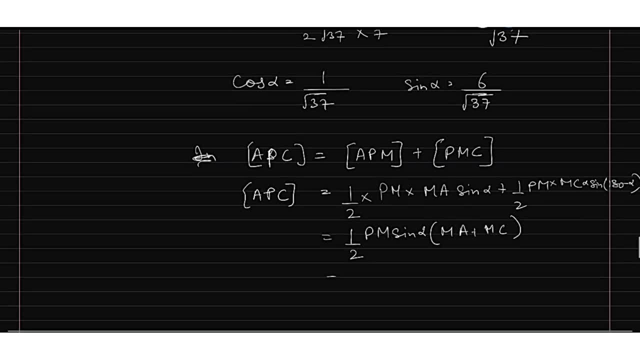 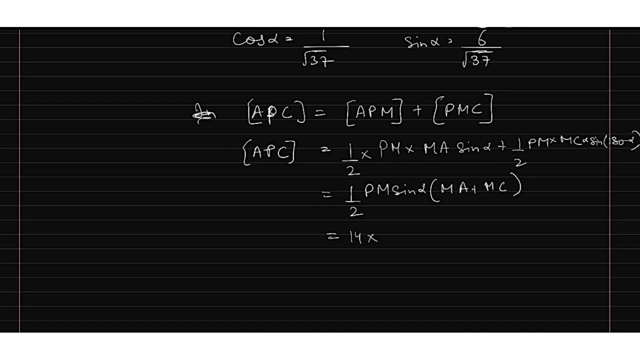 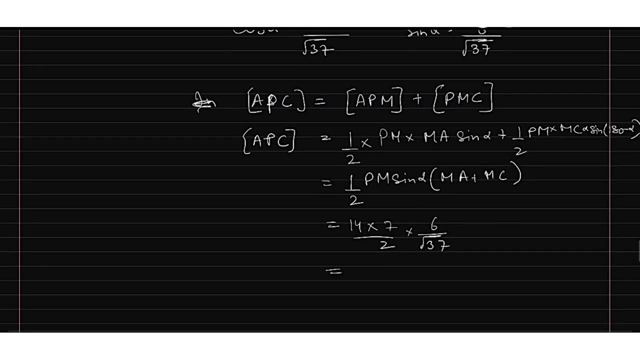 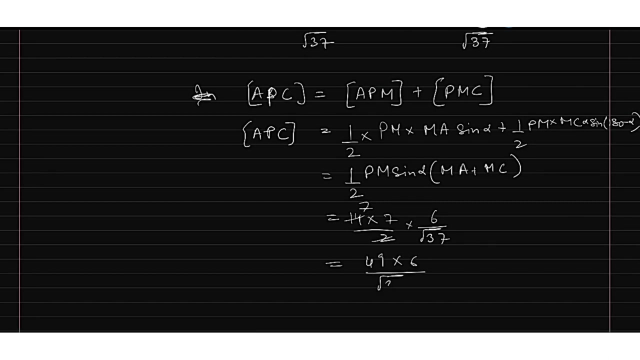 MA plus MC. What is MA plus MC? It is 14.. 14 into 7 by 2 times sine alpha, which is 6 over root 37. You can cancel this 49 into 6 over root 37. It equals 294 over root 37.. 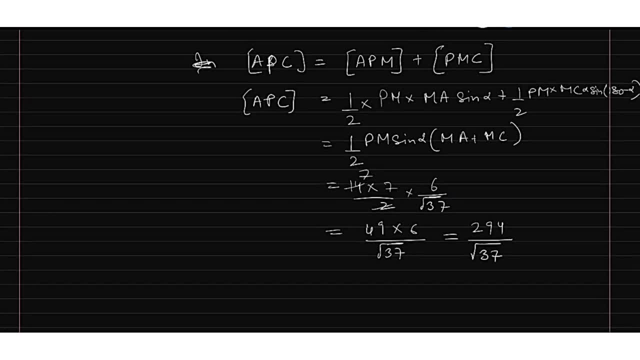 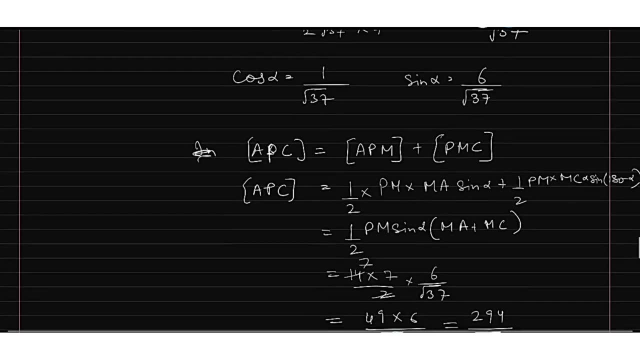 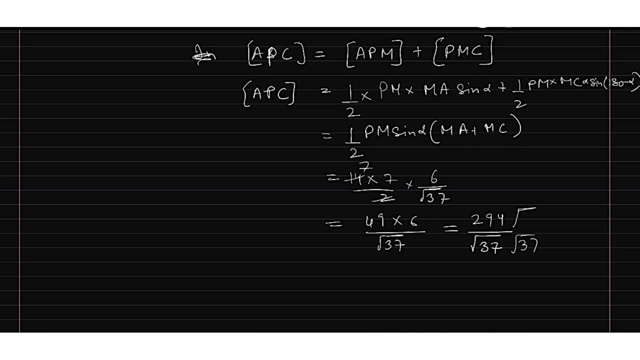 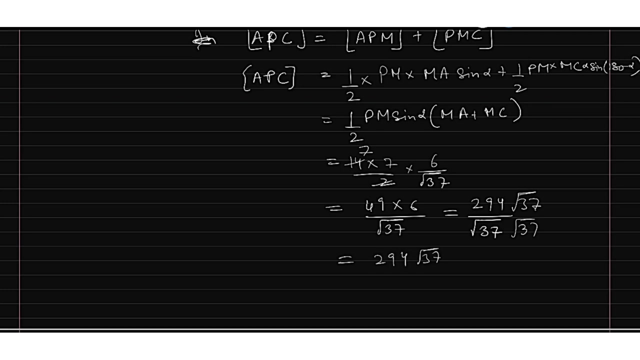 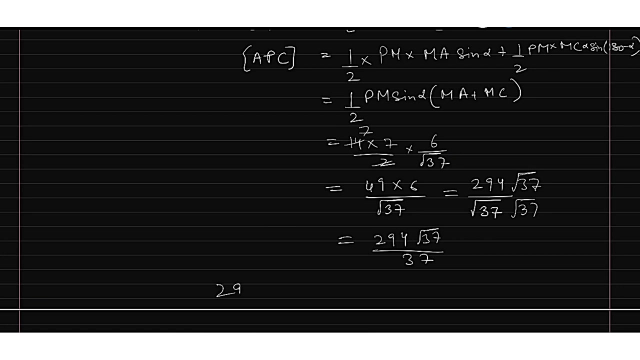 So we have to simplify this. We have to simplify it further. to make it of this form: P root Q over R, We will multiply it by root 37.. Both sides It equals 294 root 37 over 37.. So the answer is 294. 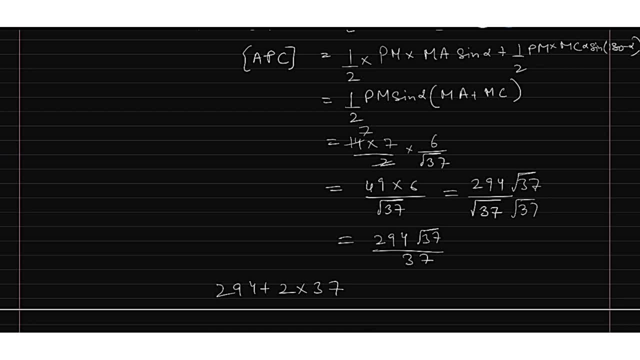 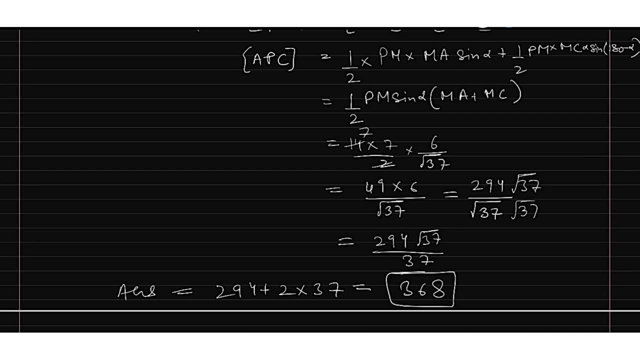 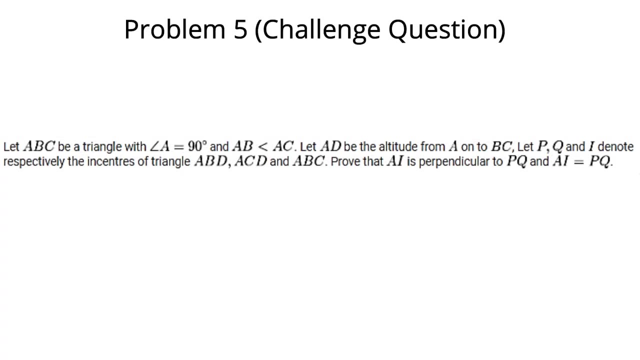 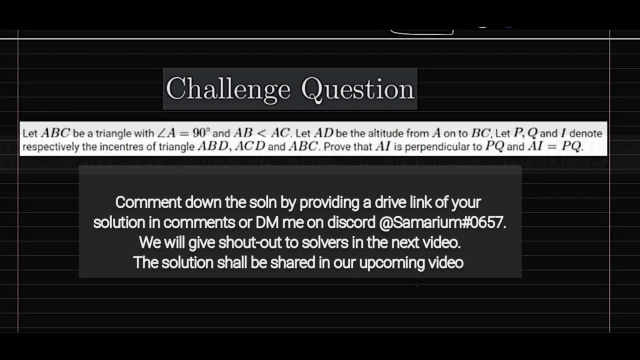 Plus 2 times 37.. Answer equals 368.. So 368 is the answer of this question. So for the fifth question there is a change. The fifth question is a challenge question. You have to comment down the solution of this question in the comments or DM me on. 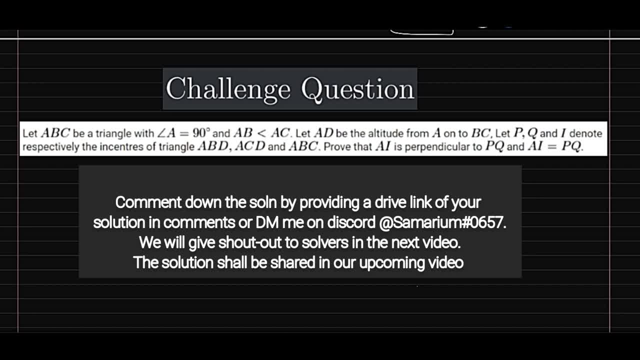 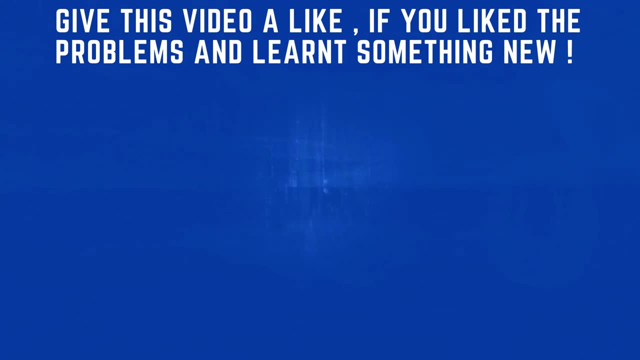 Discord on this ID. We will give shout out to the solvers of this question in the next video and the solution will be provided in the next video too. Thanks for watching. See you in the next video.